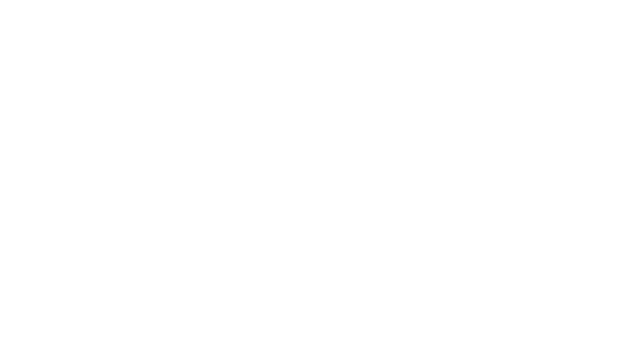 In today's video, we're going to take a look at the arrangement of electrons in atoms and see how most atoms, like the fluorine that we've shown here, have an incomplete outer shell of electrons. This is a really key point in chemistry because in order for 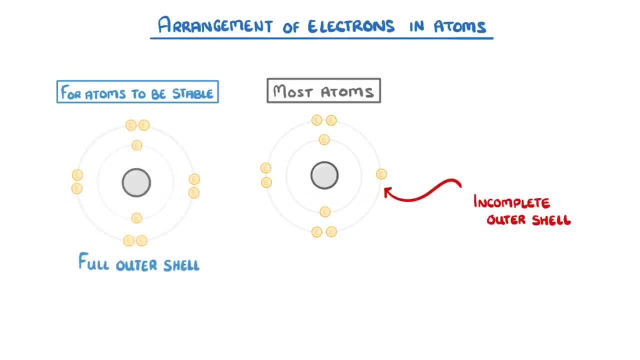 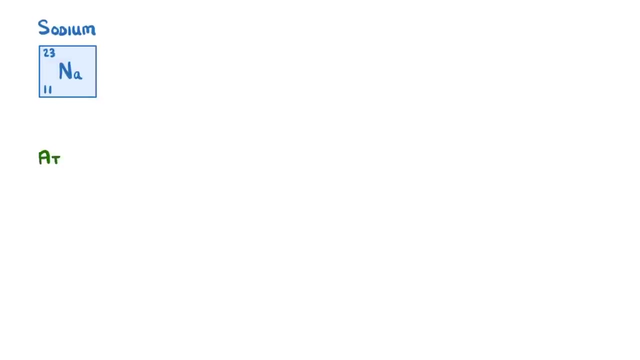 atoms to be stable, they need to have a full outer shell, And if they don't, then they'll have to react with another atom to gain or lose the electrons that they need. Let's start by drawing the electron arrangement of sodium. The fact that it has an atomic 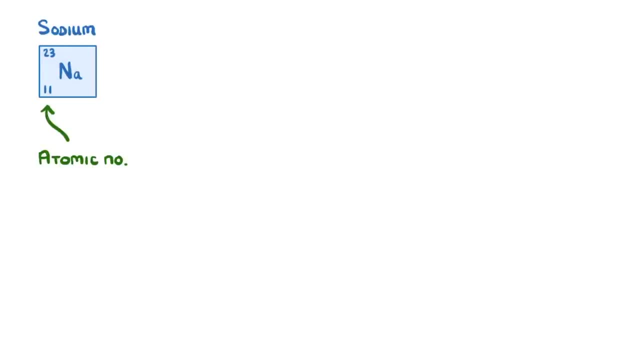 number of 11 tells us that it has 11 protons, but also that it has 11 electrons. These electrons are going to be arranged in shells around the nucleus, which we draw as rings like this, And the first one to fill is the one closest to the nucleus. 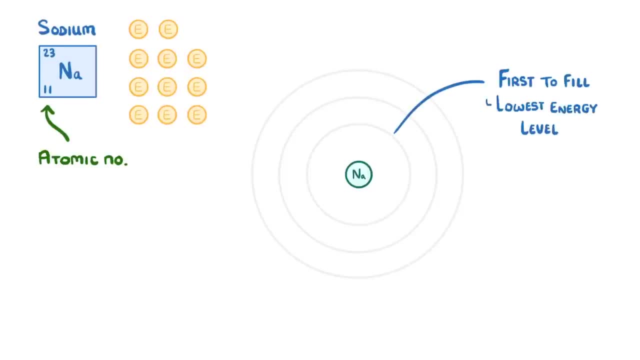 As this one will have the lowest energy level. This first shell can only hold 2 electrons. The second shell, though, can hold up to 8.. And the order in which you add them can sometimes be important. The best way to do it is to put a single electron in the top right bottom. 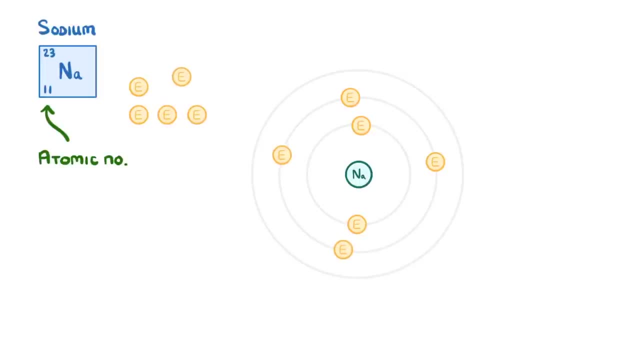 and left positions before you go round again to put a second electron in each position. This might seem a bit weird or unnecessary, but really it's not. You're just adding them in clockwise until you've either filled the shell or run out. 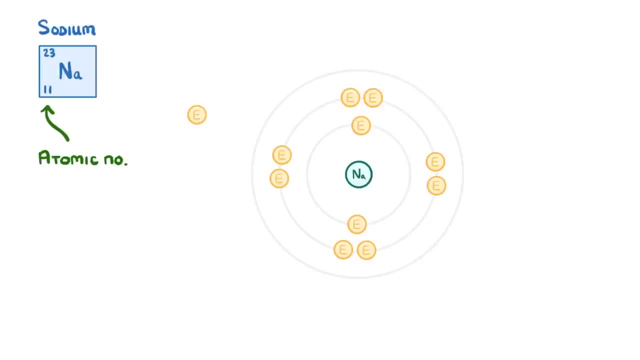 of electrons. As we still have one electron left, we put it in the third shell And, just like the second shell, the third one can hold a maximum of 8 electrons In order for atoms to be stable. their ultimate shell, meaning the one furthest from the nucleus. 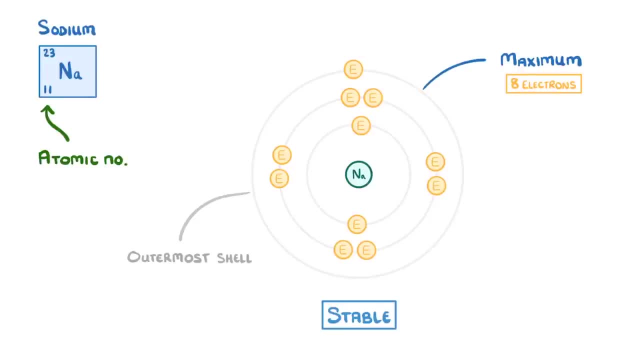 needs to be completely full. You can see here that our sodium atom only has one electron left rather than 8. So we would say that it's unstable, And all we mean by that is that it wants to react with another atom so that it can have a full outer shell. 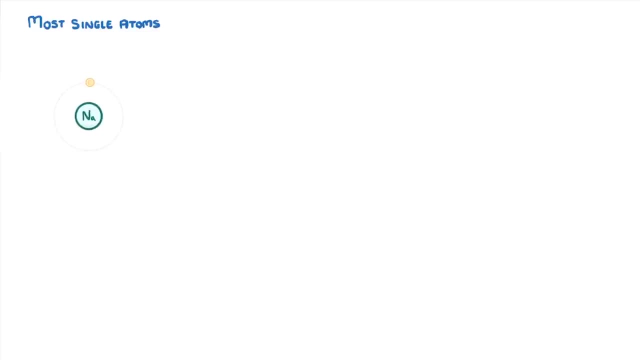 Now, most single atoms are like the sodium that we just saw. If they weren't bonded to anything, then they would have incomplete outer shells, And so, to fix this, most atoms want to react to form molecules or compounds. However, there are some exceptions to this. 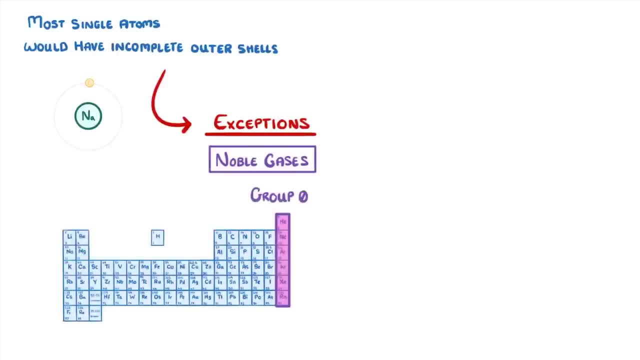 The noble gases in group 0 of the periodic table have completely full outer shells and because of this don't want to lose or gain any electrons, and so they don't react with anything. When it comes to exams, you could be asked to work out the electron arrangement of any. 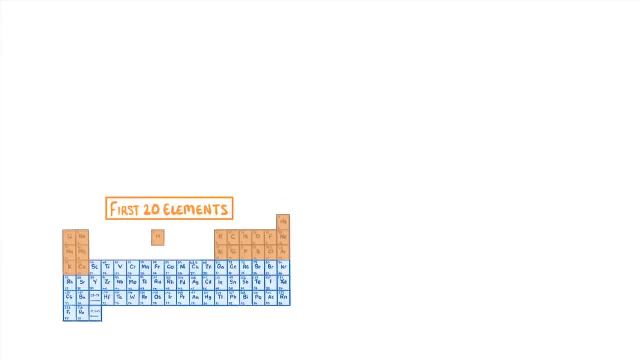 of the first 20 elements in the periodic table. For example, they could ask what is the electron structure of argon? For this we first need to find argon on the periodic table and we can see that argon has an atomic number of 18, so it must also have 18 electrons Then. 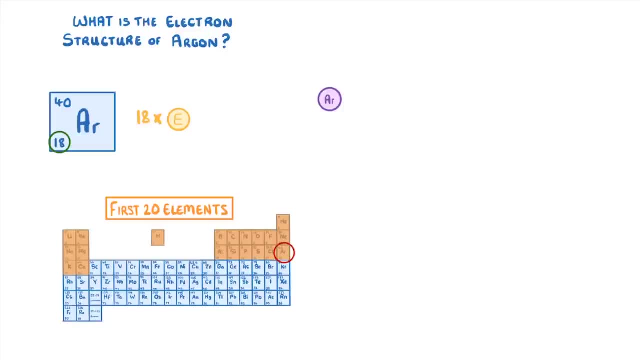 after drawing a quick nucleus, we can start to draw the shells and electrons. The third shell will have 2 electrons, the second shell will have 8, and the third shell will also have 8,, because 2 plus 8 plus 8 gives us 18.. We can also show this electron structure with: 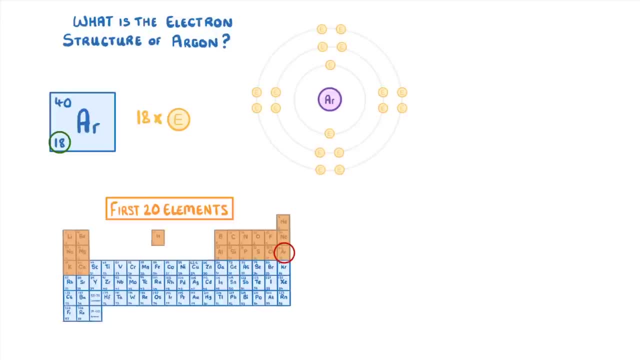 numbers, though, rather than drawing out all of these shells- and to do that we would just do 2 comma 8 comma 8, to show there's 2 electrons in the first shell, 8 in the second and 8 in the third. Another thing to point out is that when you 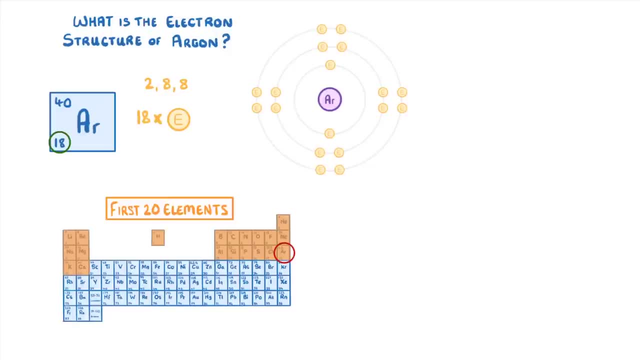 come to draw these diagrams for yourself. you would actually draw the electrons that either are just crosses, like this, or as dots, like this one. What if we were asked to do the same for calcium? Well, calcium has an atomic number of 20,. 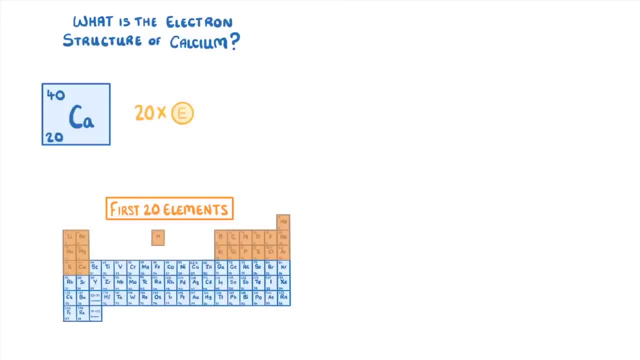 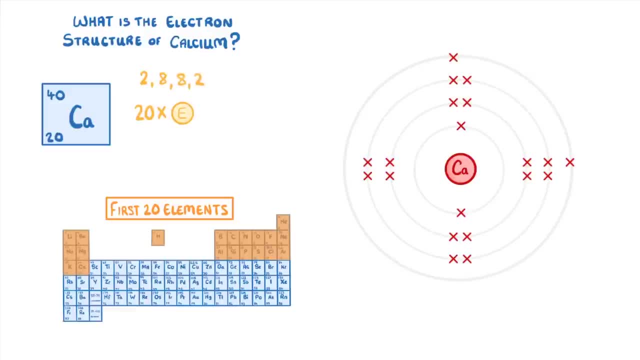 2.. As we can see from this diagram, calcium atoms aren't stable because they don't have a full outer shell. They have only 2 out of 8 possible electrons. What would help is if these two outer electrons were somehow removed. This would mean that the outermost